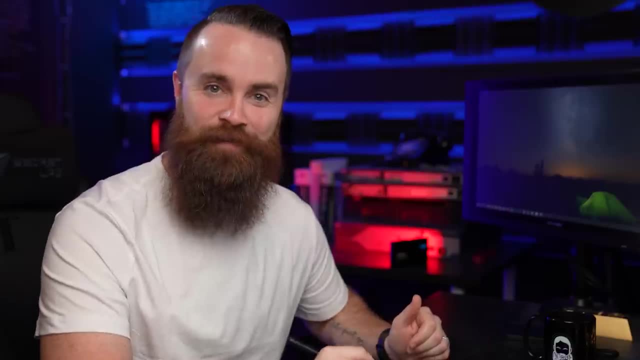 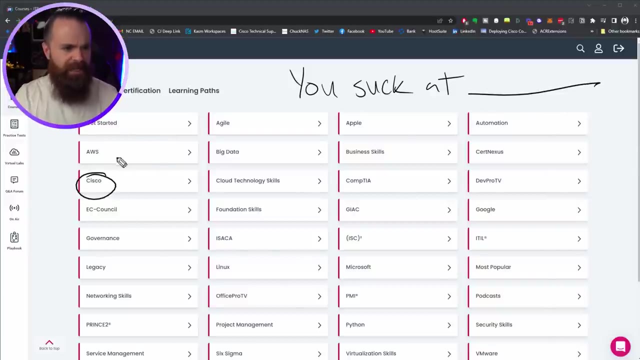 but that's okay because we have it pro TV. the sponsor of this video. fill in the blank. You suck at most things and they're going to have a course for you to learn it and stop sucking at it. from Cisco and their CCNA to AWS and their associate thing, They do it pro TV can take you. 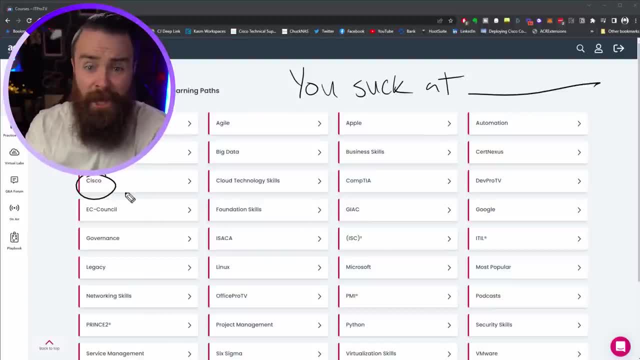 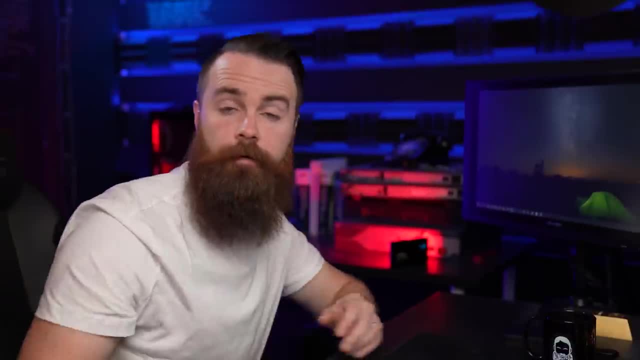 from knowing nothing in it to becoming someone who actually has a job in it, going from help desk with your comp T a plus to network engineer or cloud engineer. Oh sorry, Um, just give you an example of something that it pro TV will never make you do fall asleep because they're training. 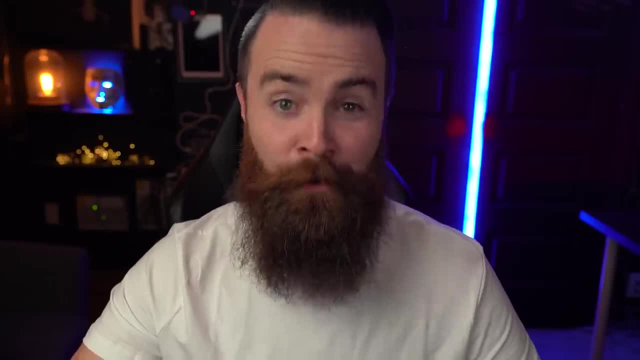 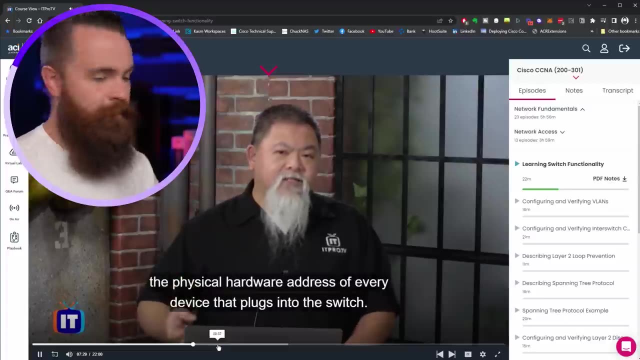 their start. That was a terrible segue, because their training is entertaining, Not boring. Honestly, it's like binge watching Netflix. What are the three F's of switch functionality, Except you're not wasting your life, and they have all the best ways for you to learn something in it. 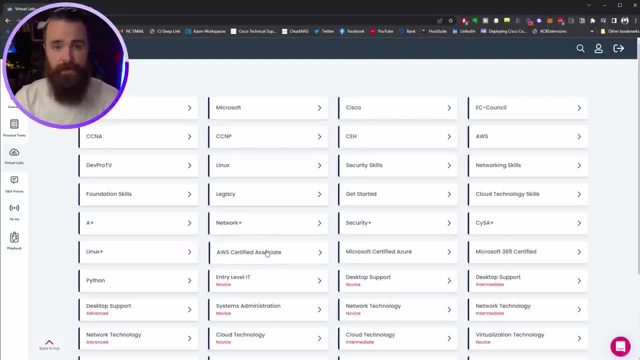 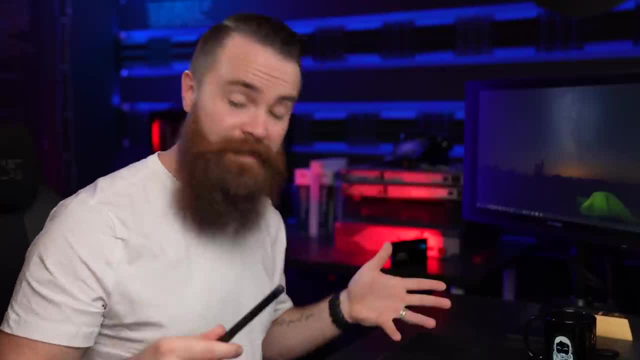 from virtual labs which are required. You have to be able to do labs for your it training and practice tests to see if you know anything and make sure you're ready for that exam. So if you want to learn it, like me and stay up to date, or just change your life and jump in it, 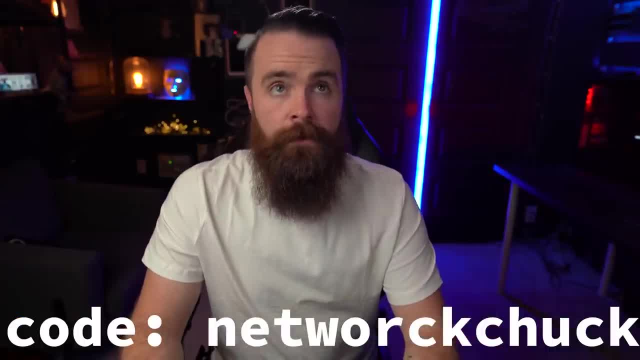 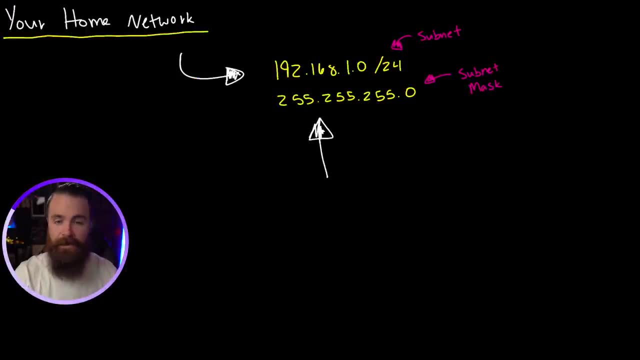 check them out, link below: use the code network Chuck and get 30% off forever. Now back to subnetting, So you can stop. I can get that for now. Now you may recall from episode five that the subnet mask here. 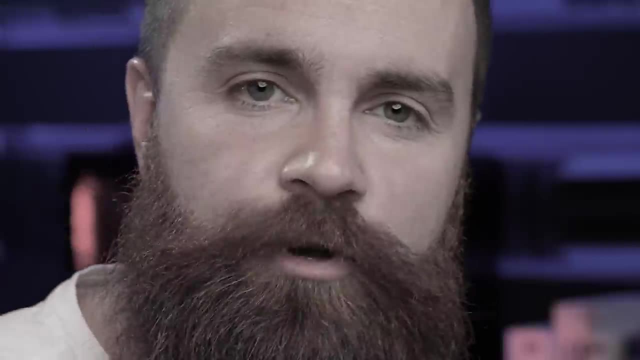 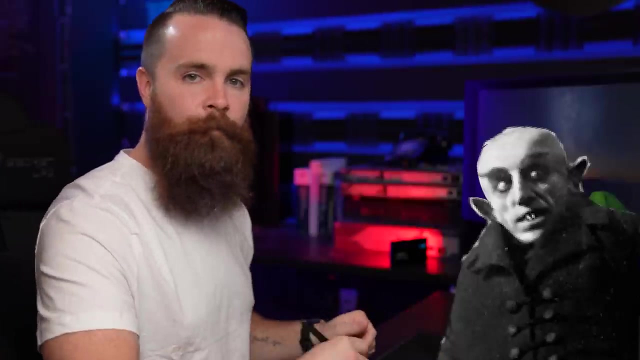 he tells us everything we need to know about the network. He whispers things to us, but to unlock his secrets we'll have to convert him to binary, using our good old buddy knows for auto. So no straw to bring in our magic chart and, with a bit of flickering lights and skills. 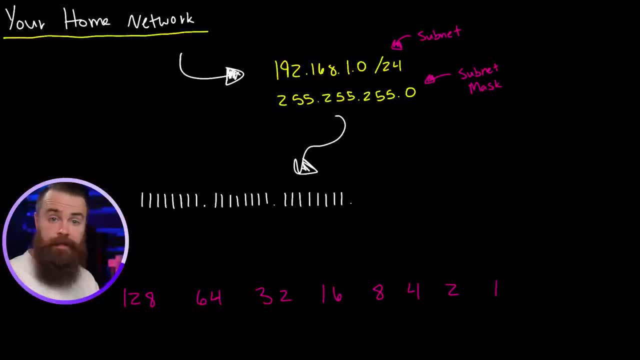 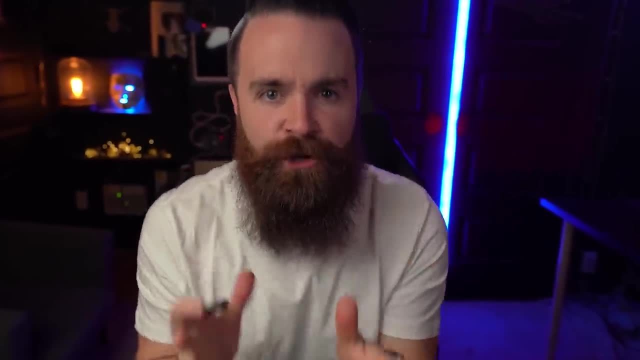 you would have learned from previous episodes. This is what our subnet mask looks like in binary, a language that computers just love. Now again the subnet mask. he's whispering things to us- deep, dark secrets- about our network, For example. if you want to learn more about the subnet mask, 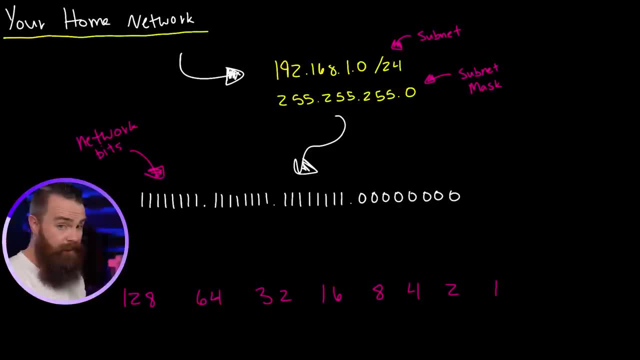 you can click on the subnet mask and you'll be able to learn everything you need to know about the subnet mask. For example, the ones are our network bits, telling us about the network, and the zeros are our host bits, telling us how many hosts can be on this network. Now here is our 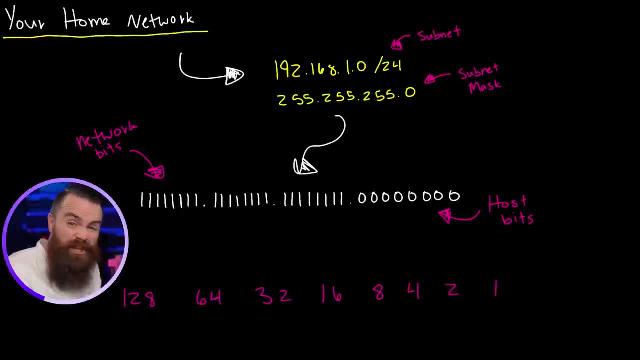 mission. We have to manipulate this subnet mask. We need to change it and break it into four networks. And here is the secret to our mission. When we need more networks, we know we need four- We need to hack the host bits. We got to flip them. We got to bring him over to the dark side. 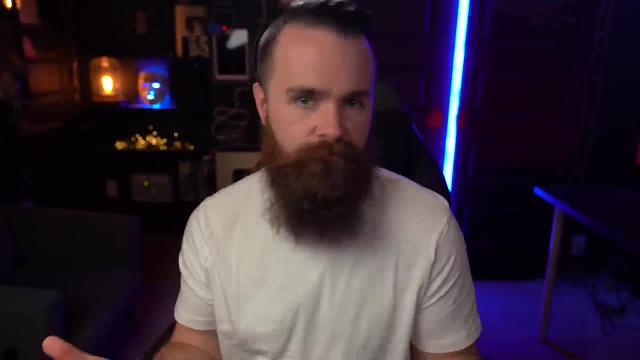 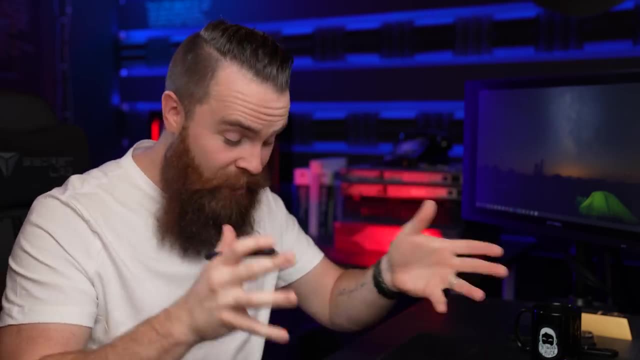 of the network bits. I don't know why the network bits of the dark side. I just felt like I should say it Felt good. So cement that into your brain real quick. When you need more networks, you need more bits, And the only way you can get more bits is by hacking them or stealing them. 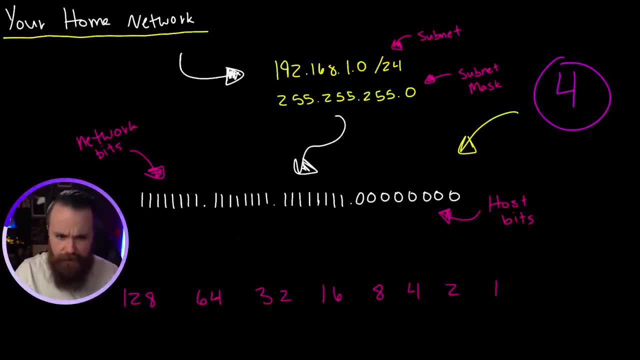 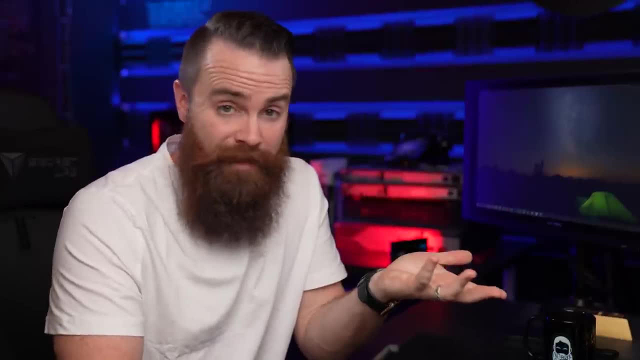 from the host bits. But how many of the host bits do we need to create four networks. That's where a new friend comes in, because I bet you didn't know that knows fraud too. He has a brother now where knows fraud too. helps us with decimal to binary conversion. His brother knows fraud too. 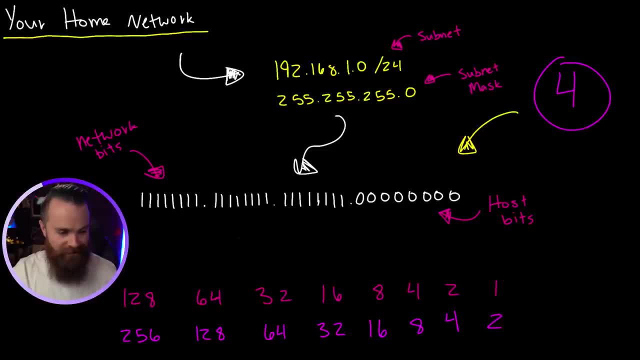 helps us with this problem And he even has his own chart. Check this out. This is the no spraw to chart, because, notice, every single number in that chart is just the number in knows fraud to start Time, Sue. So we say, Hey, no fraud too, We need four networks. And he says: 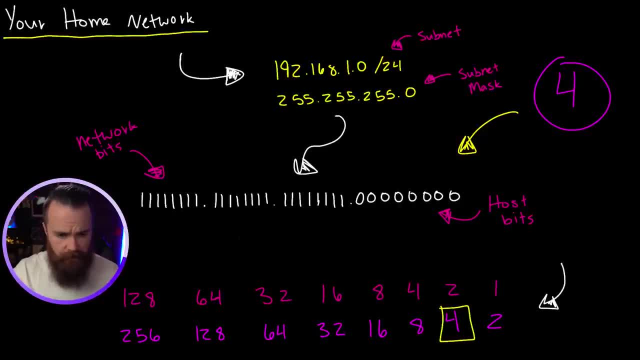 okay, let me see here, Here's four, And that took us one, two bits to get there. And that's exactly how many bits, how many host bits, we have to hack and steal to create four networks out of our existing network. Now, just to hit this home a little bit, What if I asked you: Hey, I need you. 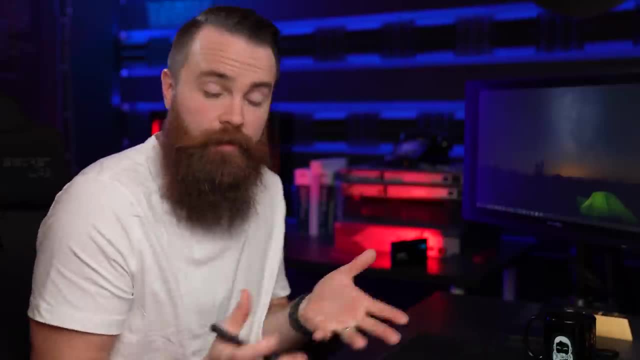 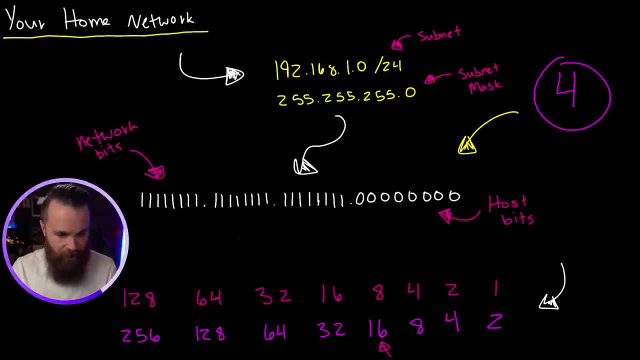 to make 17. networks out of our existing network. Well, you would tell Nosferatu: Hey, I need 17.. So Nosferatu will look at his chart and go, Hmm, All right, 16.. That's not quite enough, We need 17.. So I gotta jump to the next one, 32.. 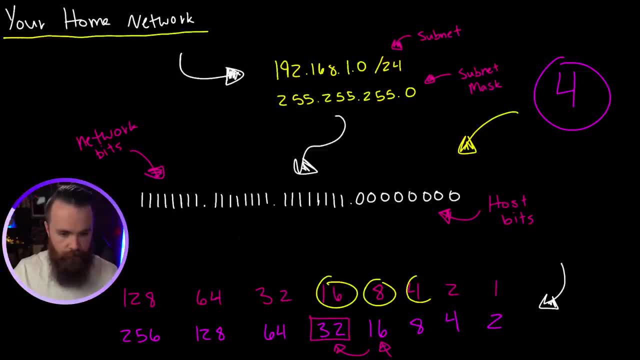 And how many bits did we need to make? 32, 1,, 2,, 3,, 4, 5.. So in that scenario, to have at least 17 networks, we would need to use five bits. We have to steal five bits from the host. But in our example, 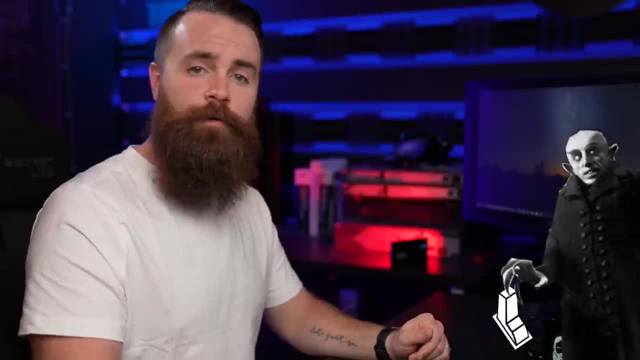 all we need is four, which only required two bits. Thank you, Nosferatu. And now that we know how many we need to hack, let's go ahead and hack them. Let's flip them, bring them over to the dark side. 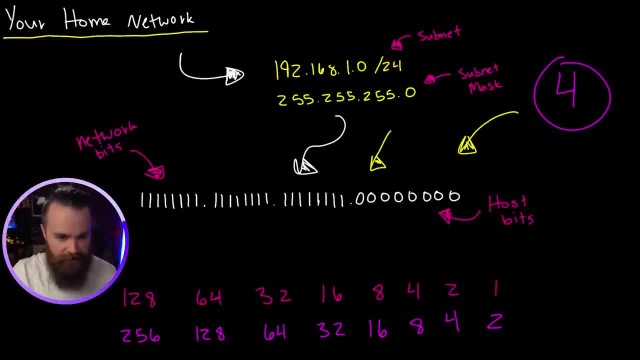 So, starting at the beginning of our host bits, we'll hack two bits, hacked, hacked and we'll flip them over to the dark side. Gotcha Host bits. Now that right, there is our new subnet mask. You just submitted a network from one network into four networks. 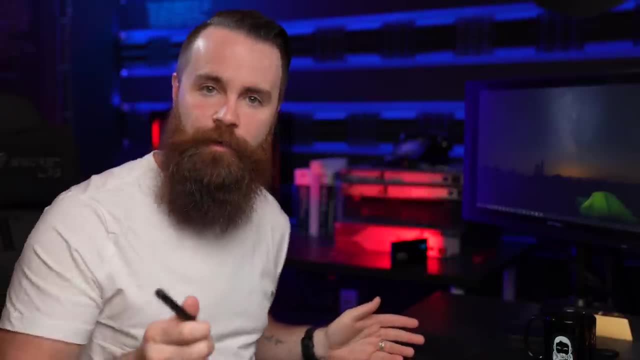 Now we're not quite done yet. Our mask is still in binary. Let's use Nosferatu, You know the first one to convert our mask back into decimal. We know that all ones are two, five, five, because all bits are on. 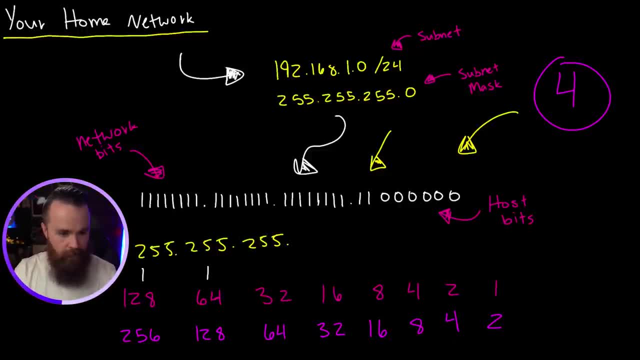 Okay, And in our fourth octa we can see that the first two bits are on and the rest are off. And if we add one 28 to 64,, what do we get? One 92. That's our new mask. 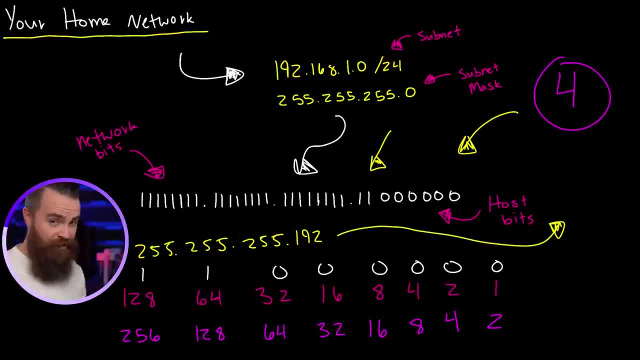 And if we were to write that inside our notation, which is simply just counting all the network bits in our mask? we get eight, 16,, 24,, 25,, 26.. We have a slash 26 network. How cool is that. And there it is: Our first network, new and shiny. 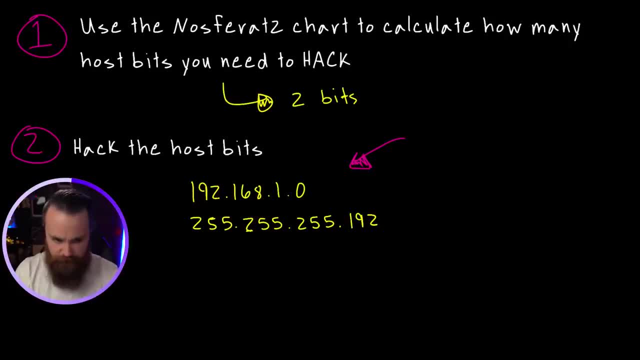 So cool, But hold up How many hosts are in this network. Like we can see, the first IP address in the network is this, but where does it end? What's the broadcast address? How do we find that? How do we find the resulting networks and what their ranges are? 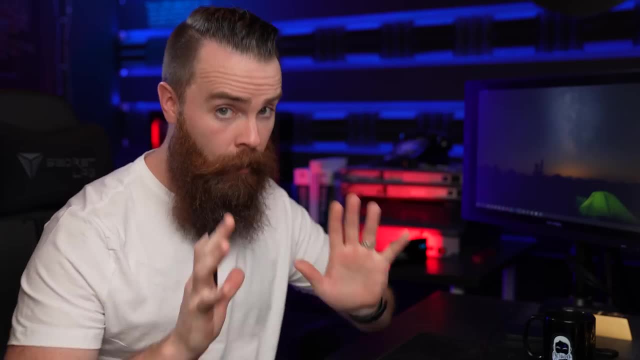 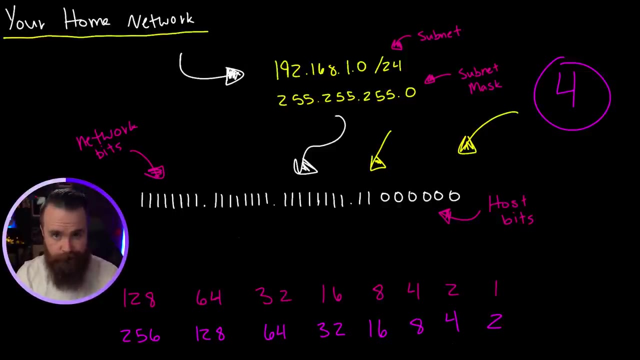 We need to find the increment, which is super easy, by the way. Now watch how hard this is. I'm totally kidding. Watch this. The increment is simply the last network bit we have. So, looking at our binary here and our subnet mask, there it is. 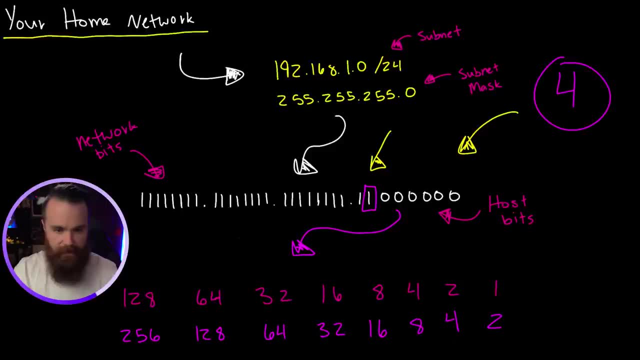 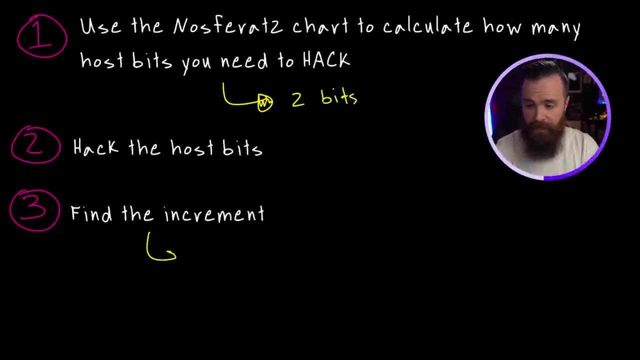 That's our increment. And if it were to draw our last octet on our chart here, our increment is right. here And there it is. And decimal 64 is our increment. 64 is what we'll use to determine the size of our networks and what the 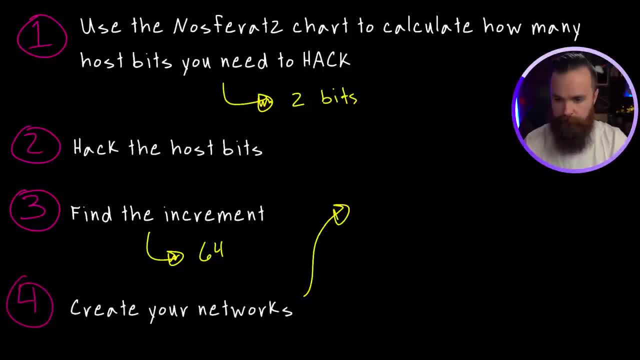 ranges are. Let's go ahead and do it right now. Let's start with our first network, Of course, obviously one nine, two dot, one, six, eight dot, one dot zero through one nine, two, one six eight dot, one dot. This might trip you up a little bit. 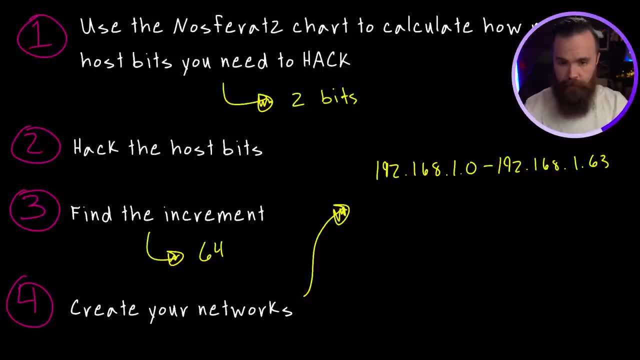 63, not 64, because, remember, we're including the zero. The zero is still An address. that right. there is our first range, Our first network. Let's do the next one. It'll pick up right where the last one leaves off. 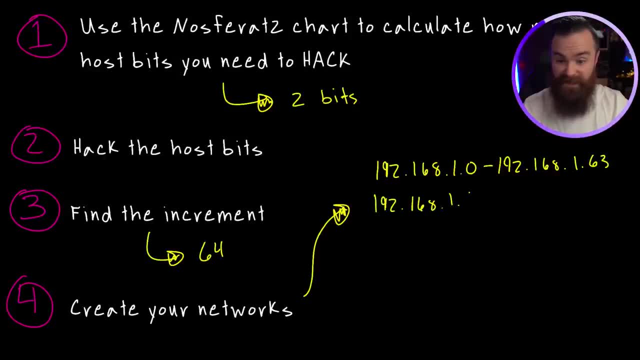 One, nine, two dot one, six, eight dot one, dot 64 through. And if you add 64 to 64,, what do you get? 128. But remember, we have to include 64. So the number will actually be one, 27.. Now I think you got it. 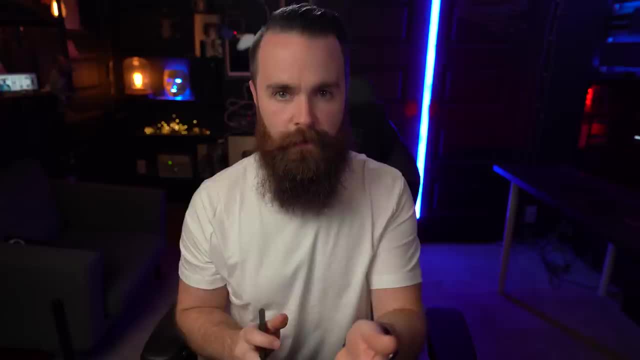 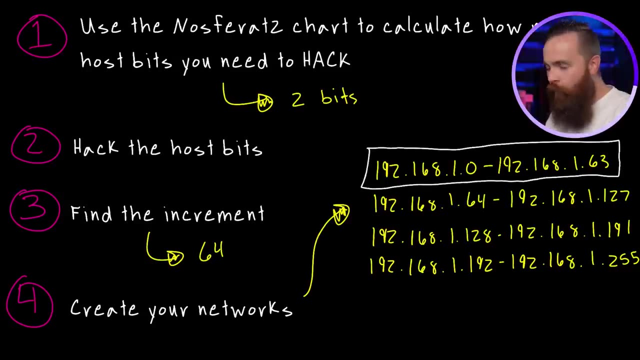 I'll fill out the rest real quick. Actually, you know, pause the video. You fill it out, boss, unpause. And there they are, Our four Networks that we created out of one network using the power of subnetting. Each of these networks will have a subnet mask of two, five, five. 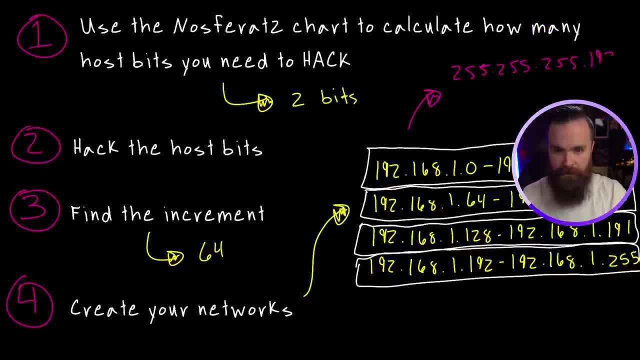 two five five, two five, five, dot one, 92 or slash 26.. And a quick quiz to test your knowledge: How many hosts are in each of these networks? Keeping in mind that we now have less host bits- right, We borrowed some- 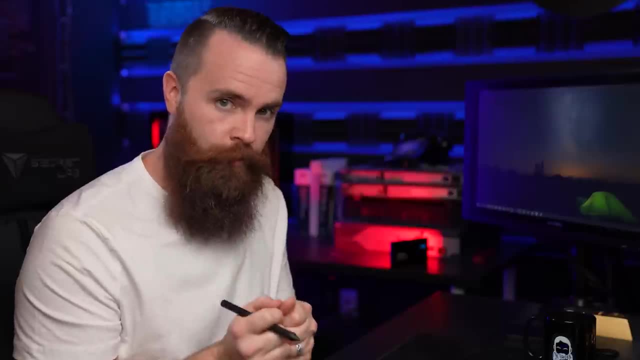 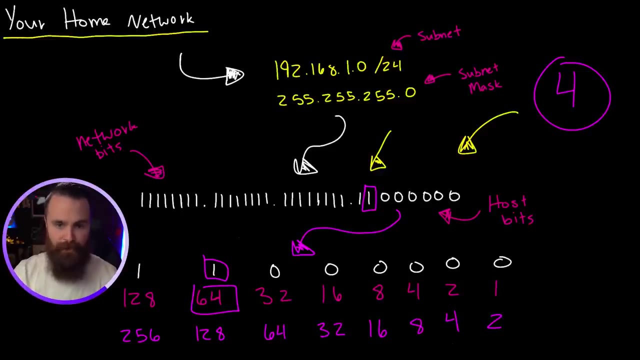 we hacked some, we stole them, So now there's less hosts available in each network. Now, if you look at our increment, it's probably painfully obvious, right? But the formula from our past video still works, If you recall, to figure out how many hosts are available in any given network. 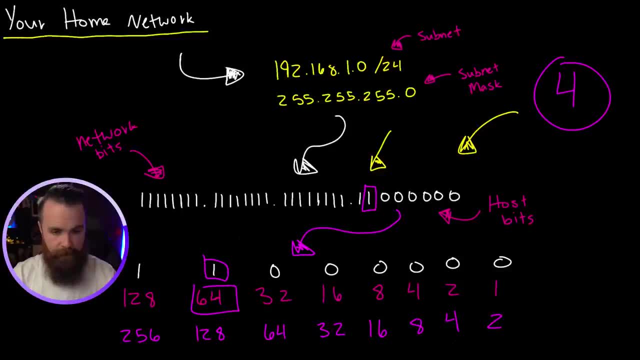 we can look at our subnet mask in binary and count the number of host bits. How many are there? One, two, three, four, five, six. There are six host bits in this network And the formula will be two to the power of host bits, which is six. 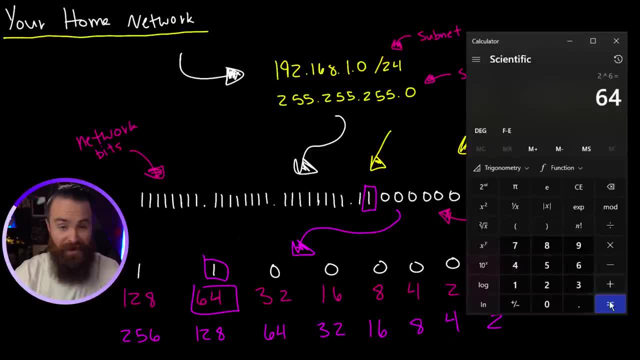 which we could use a calculator to figure that out: Two to the power of six, which is our increment. Or we could simply ask Nosferatu looking at our six bit: one, two, three, four, five, six, And then, of course, 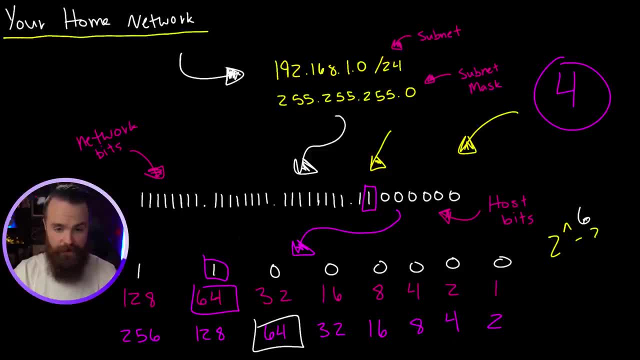 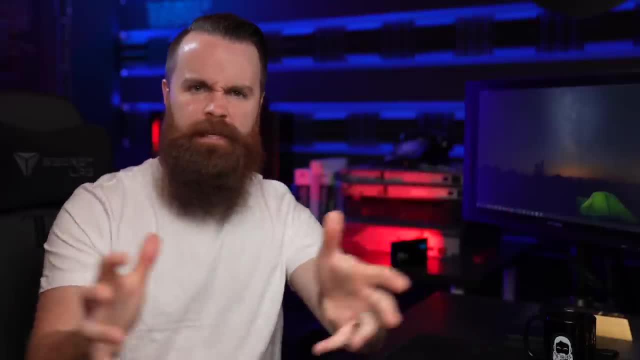 if we account for the subnet address and the broadcast address, subtracting two, we get 62 usable addresses in our network. So when someone says: Hey, I need you to take this network and break it up into a million pieces, like maybe six or seven or 12,. 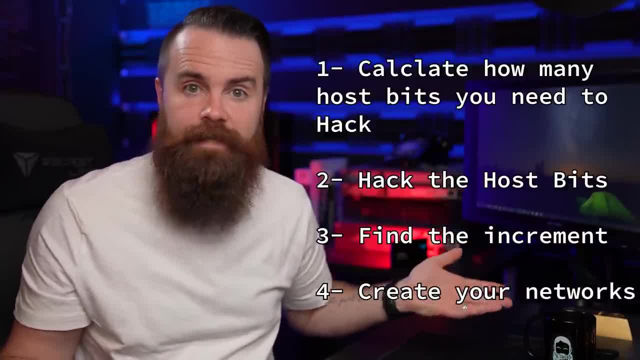 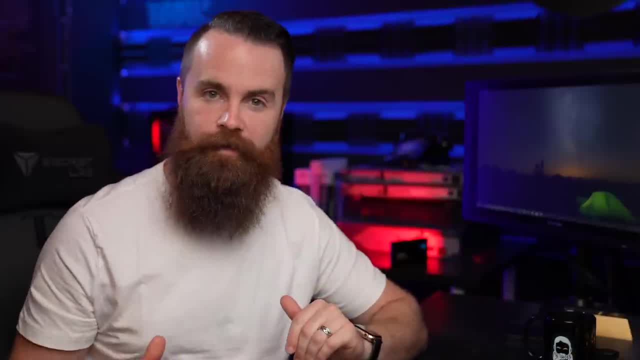 you can take these four steps and do it like it's awesome. In fact, I want you to do it right now. Here's your homework. Instead of four, I want you to do five networks. take that same network in this video and convert it into five. 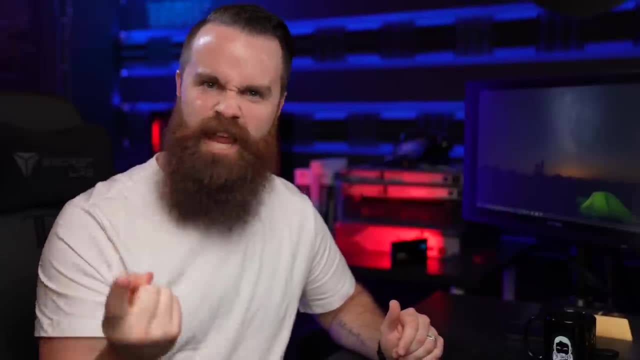 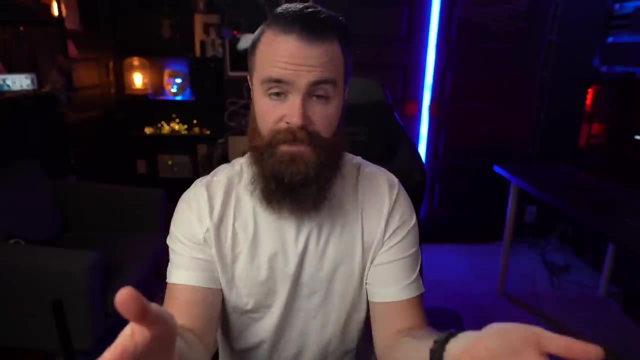 I want you to paste the answer below the subnet mask. I want to see the regular version and side of notation And I want to see the ranges. Let's see what you got. Now I have good news: No matter what type of network you encounter, these four steps will work. 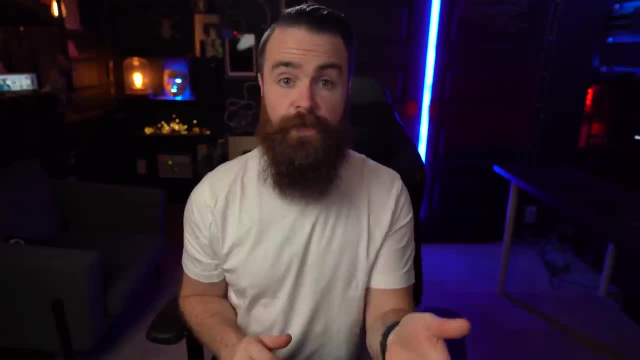 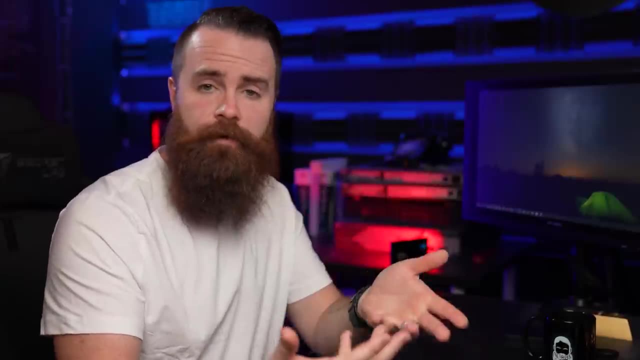 If someone gives you a network requirement, we need this many networks. You can figure it out. but I will say this: We've been doing a class C address, one nine, two, one, six, six. It might feel a little weird when you do a class B or a class a address. 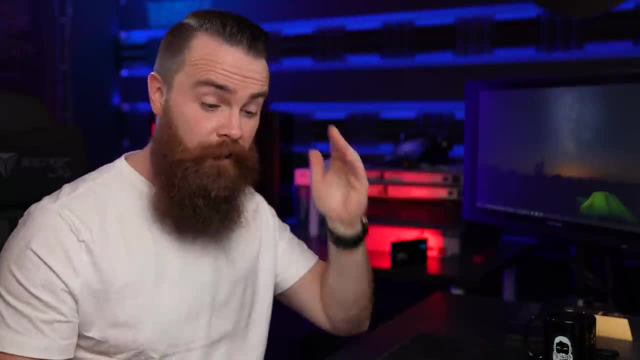 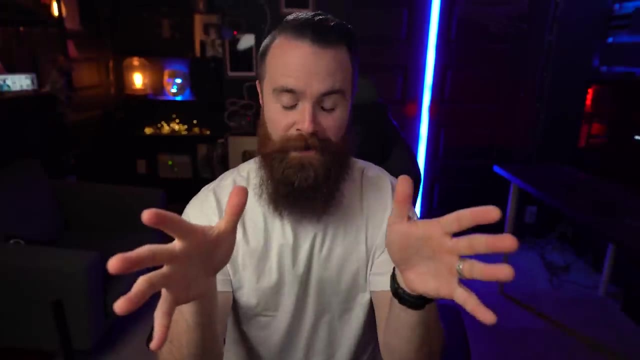 Now it will be the same. It just might feel weird. So if you want some extra practice with the other classes of addresses, I've got a link below. We've got some extra training on this and some extra practice. but I do want you to take a moment and just think like 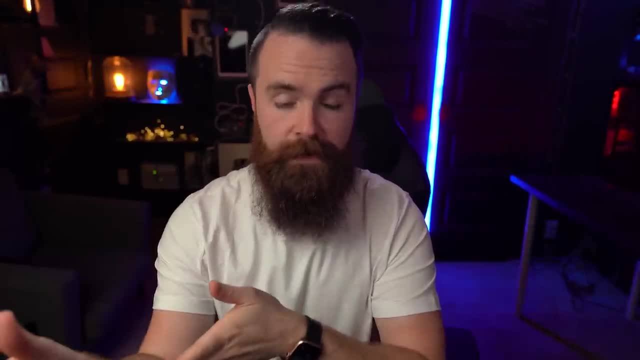 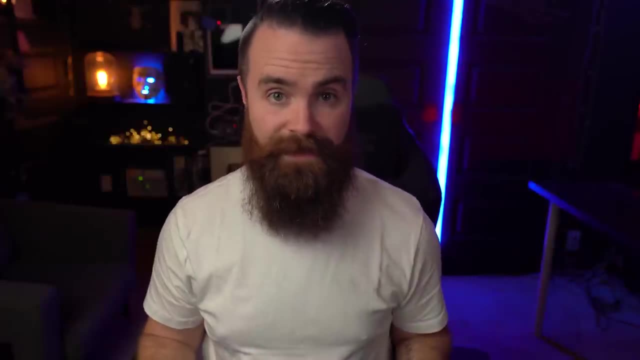 okay, here we are at episode six and our you suck at subnetting series And you now have just learned how to subnet a network, to take a network and make it in too many networks, And that's a pretty stinking big deal. You've come a long way and this is a skill you will use, and almost no every.